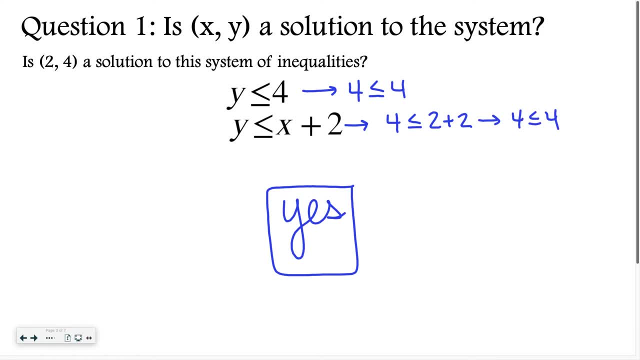 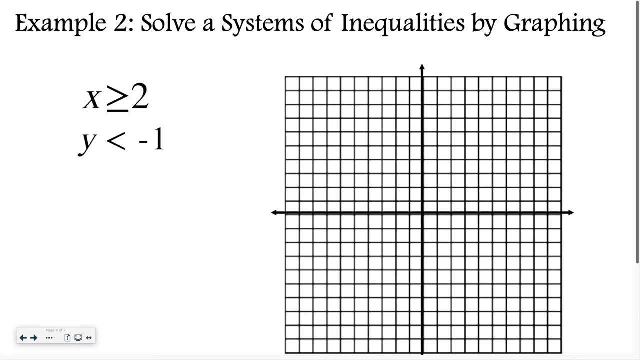 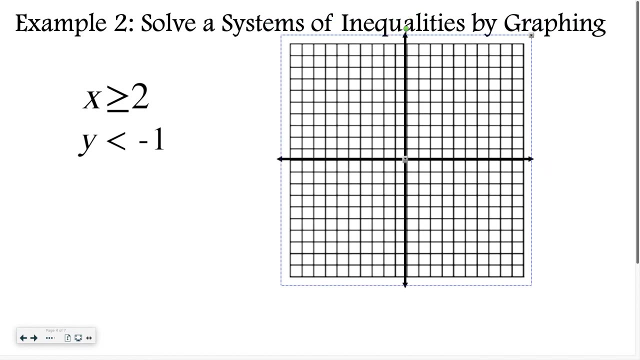 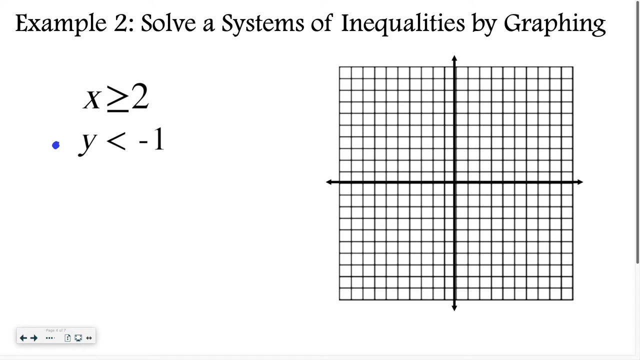 I'm more than happy to help you. So your first assignment on IXL is going to be exactly like this. I recommend doing this: IXL skill first- okay. Now example two: solve the systems of inequalities by graphing. Okay, so what I'm going to do is I'm going to assign colors to each of my graphs. 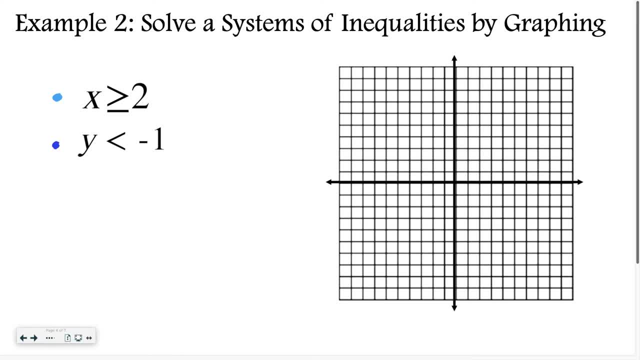 So hopefully those two colors are somewhat easy to differentiate. Now I'm going to graph that X is greater than or equal to two. So this is going to be a solid line, And then the Y is less than a negative one. That's going to be dashed line. 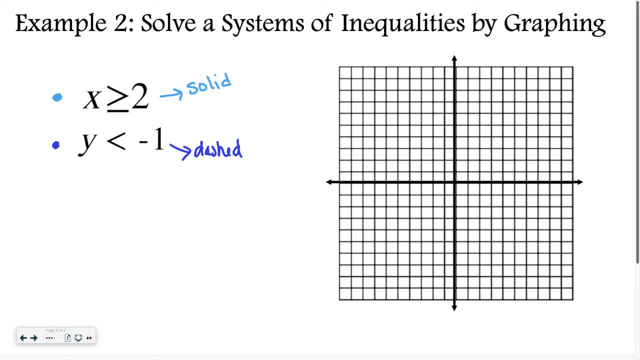 Sometimes students do better if they immediately write whether it's solid or dashed, because that's an easy thing to forget and lose points on your answer for that. All right, so X is greater than or equal to two. So where X equals two on the X-axis. so this is my X, here is two. 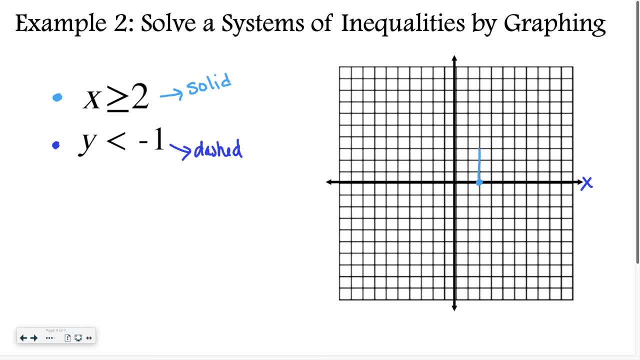 And then X equals two along this entire line. So I'm going to do a solid line going straight up and down. okay, Then I'm saying: X is greater than or equal to two. So that greater than. where does X start to get bigger? 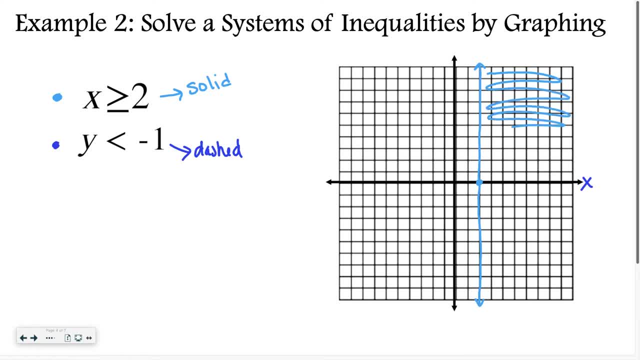 X starts to get bigger on this side. Okay, So I'm going to do a solid line of my line. okay, So I'm going to try to shade it in, make it really obvious where we are talking about. okay, So I have that shaded in. 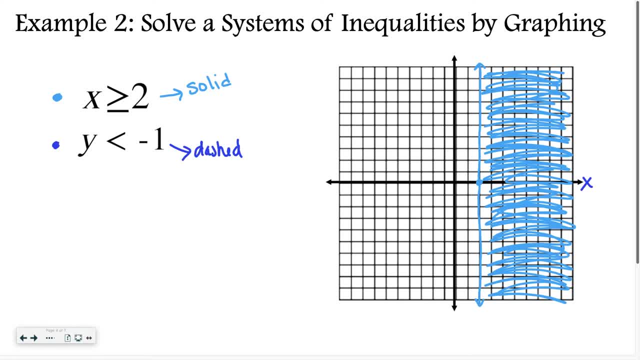 Now Y is less than negative one. Y-axis is right here, Y is negative, one is right here, And I'm going to do a dashed Line at: Y equals negative one and then Y is less than negative one. So that's going to be everything below. 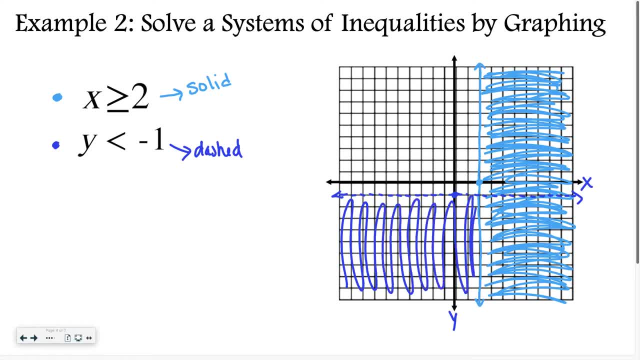 So I would go like this: Okay, so you can see, it starts to get a little messy when you are writing your answers or putting your answers into IXL. It works pretty much the same as yesterday, except that Shading the solution is where they overlap. 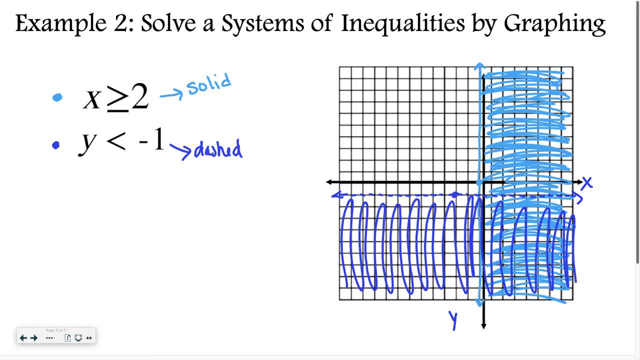 Okay, So the solution only includes- oops, did not mean to do that. The solution only includes the overlap, So you would not include any of this other shading because that is not considered part of your answer. Now, some of you might need to have that shading. 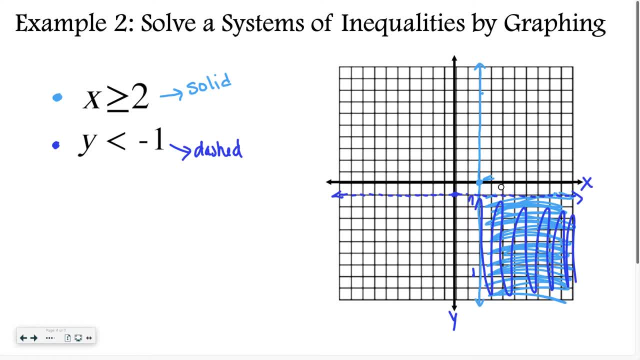 You might want to have that shading. Okay, that shading there, just to help you keep track. And, on your test, I'm okay with you using different colors and having all of that shading on there. However, on iExcel, when you're doing your, 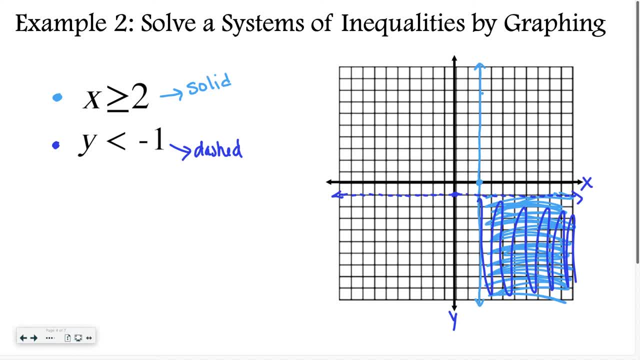 assignment. it's only going to let you shade in this one little box, because this is your solution. Your solution is the overlap And on your test, like I said, you're welcome to leave all of that shading that I had on there, And then you could just draw an arrow and say which part is your. 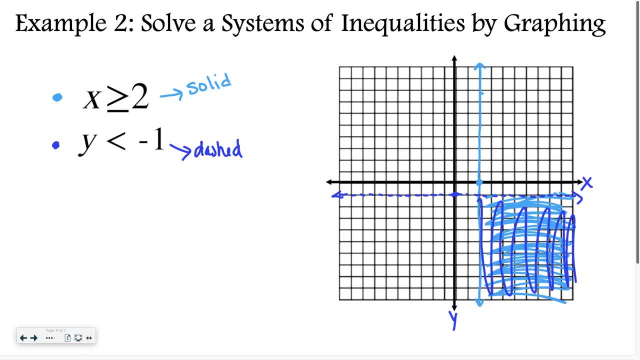 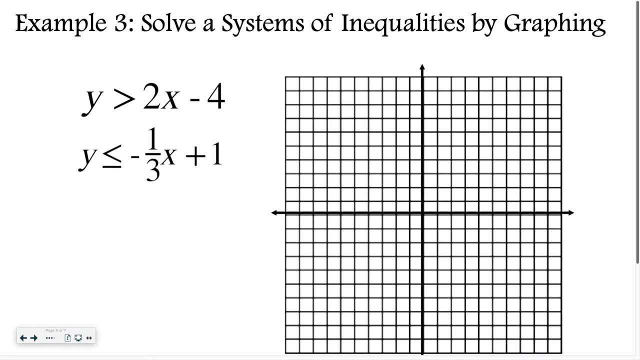 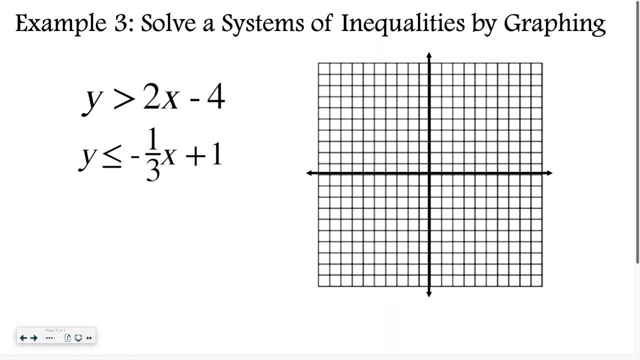 overlap your solution or use like a third color, But for iExcel you would only be able to highlight that one little section. Okay, let's try another one. I know these really start to look confusing. I know they are not always the easiest thing to learn, And if it makes sense, 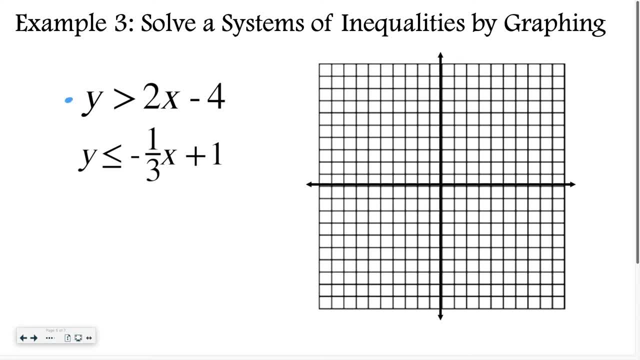 awesome, That is fantastic. It just doesn't always happen for everyone, And that's okay. So we have: y is greater than 2x minus 4.. So my y-intercept is a negative 4. My slope is 2. And this is going to be a dashed line. So I'm going to go up 2 over 1,, up 2 over 1,. 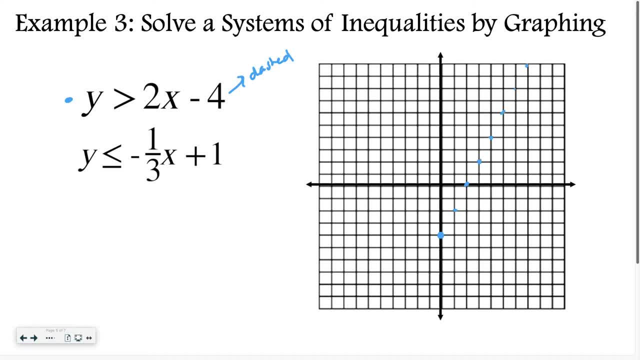 up 2 over 1.. I like to put as many dots as possible to help me keep my line straight, And since it's dashed, I'm just going to go like this. And voila, I have my line. Now remember to figure out which part I would shade. 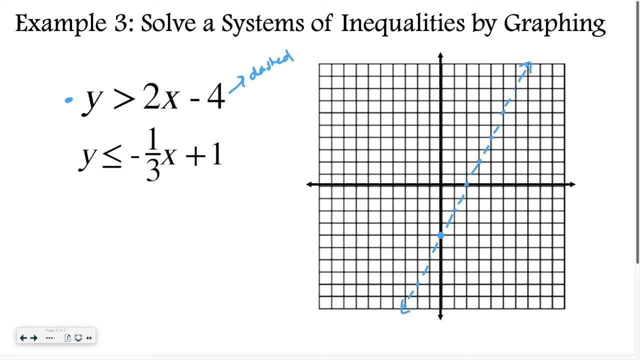 I would plug in a point. Remember you can pick any point that is not on your line. So I'm going to pick 0, 0.. If I plug 0 in is 0 greater than 2 times 0 would be 0 minus 4.. 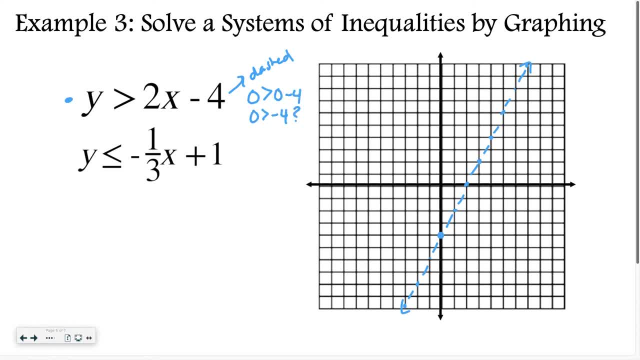 So is 0 greater than negative 4? Yes, So I know I'm going to shade all of this, because 0, 0 is on this side of the line. Okay, Now for this next one. the next line, I have a solid line because it has the or equal to My y-intercept is 1.. 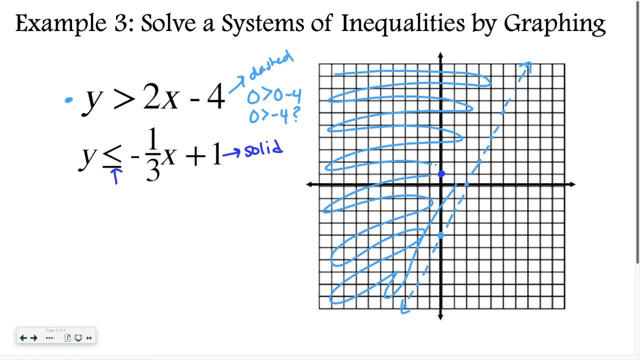 My slope is a negative 1 third. So I'm going to go down 1 over 3, down 1 over 3, down 1 over 3.. Or I could go up 1, left 3.. Up 1, left 3.. Up 1, left- 3.. And again I'm going to do a solid line through those dots. 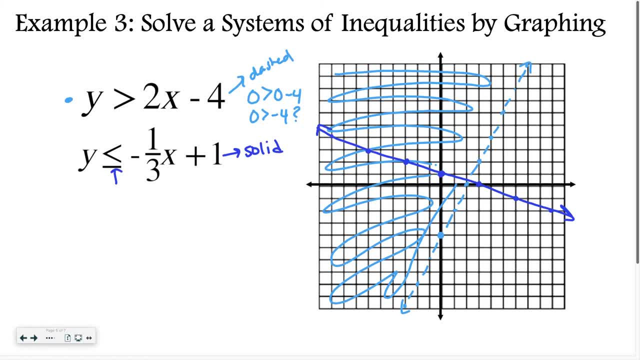 And now I need to figure out: am I going to shade above or below this line? So this line doesn't go through 0, 0 either. So I'm going to plug that point in. Is 0, that was a bad 0. Let me try again. Is 0 less than negative 1 third times 0 is just 0 plus 1.. 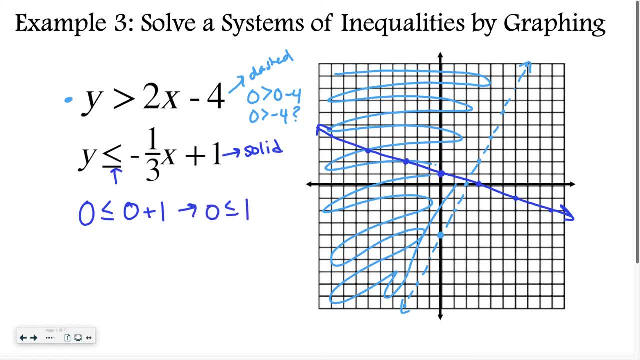 So is 0 less than 1? Yes, So I'm going to go to this line that I just drew in. I'm going to shade everything on the 0, 0 side, So that would be everything down below this line, But I'm going to make my life a little bit easier. 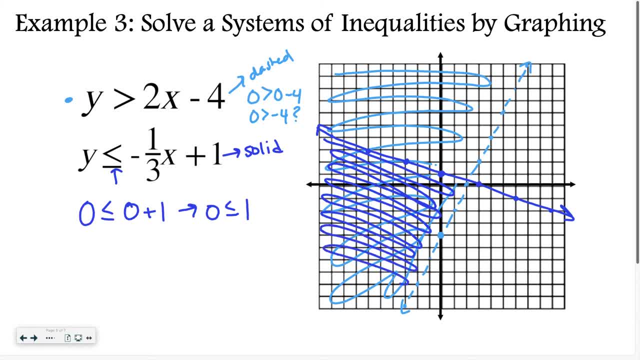 And I'm only going to shade in the overlap part, Okay, Because that's all that IXL will let me put in. So I would erase the rest of that And this would be my solution, Okay, So sometimes when you're doing IXL, it's actually easier to do it on paper. 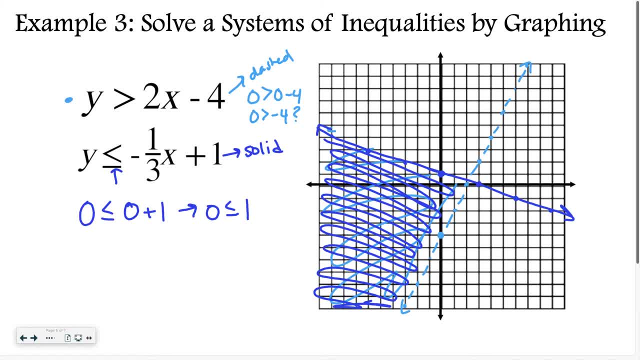 So that way you can see what parts you're shading and then put it into IXL. In the past this has taken students a lot of like a lot of questions, a lot of tries to get to the one ribbon, And the students that take the time to write it down like this usually end up doing fewer questions. 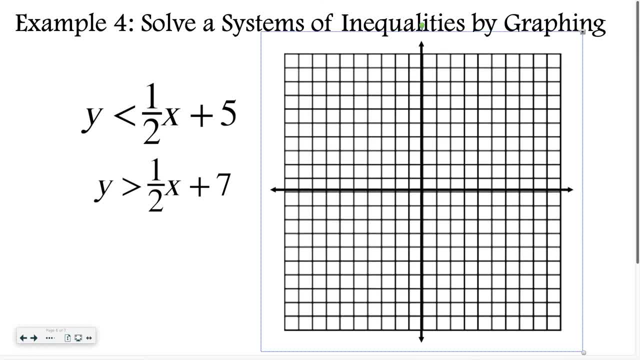 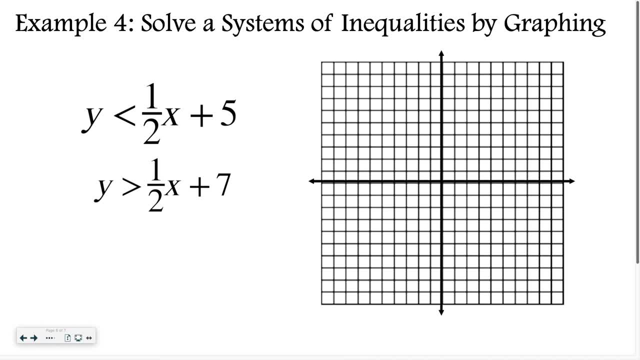 Because they end up just doing better on the problems. So I highly recommend. I gave a bunch of you some graph paper last week. I recommend using that. Then this top equation: this is our last one for today. This is going to be a dashed line And my Y intercept is 5.. 1,, 2,, 3,, 4, 5.. My slope is 1 half. 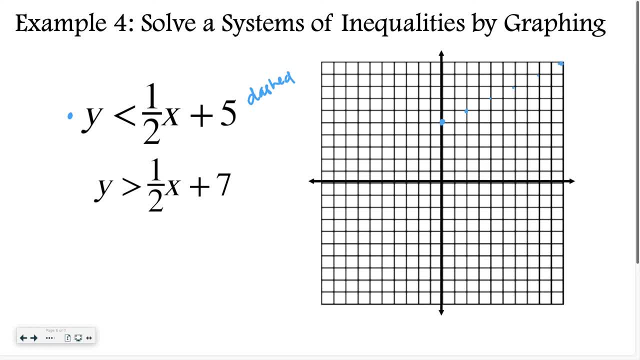 So up, 1, over 2.. Down, 1. Left 2.. And then this is dashed. So, voila, There's that, And if I plug, I just like to do 0 of 0.. If I plug 0 in, I have 0 is less than 1, half times 0 is 0. 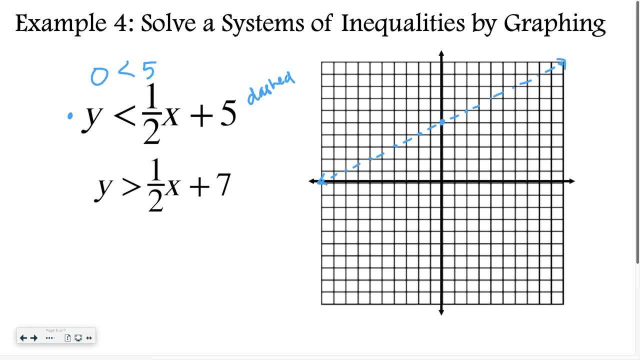 So 0 is less than 5.. That's everything below here. Okay, So I'm going to shade that all in. Okay, Then for the second one. that's another dashed line. This time my Y intercept is at 7.. My slope is 1 half. 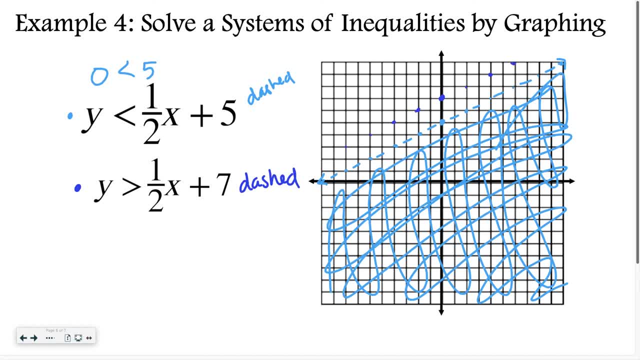 So again I can put my dots there to make it a little easier to draw in. And then if I plug 0 in, 0 is greater than 1 half times 0 is 0. Plus 7. So 0 is greater than 7.. 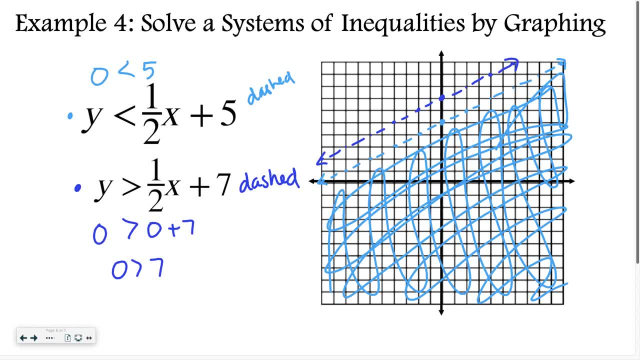 Which is not true. So I'm not going to shade the side of the line that has 0, 0. I'm going to shade the other side of that line. So this time maybe you can see that none of our shading overlaps. 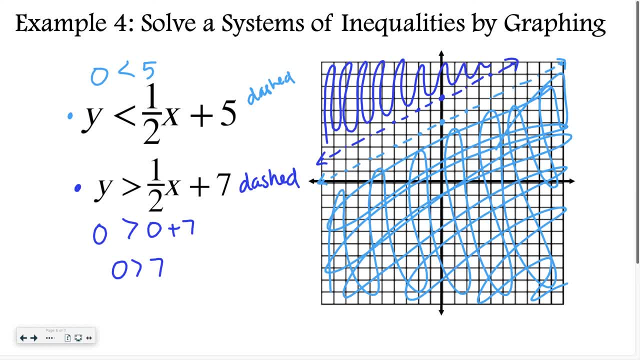 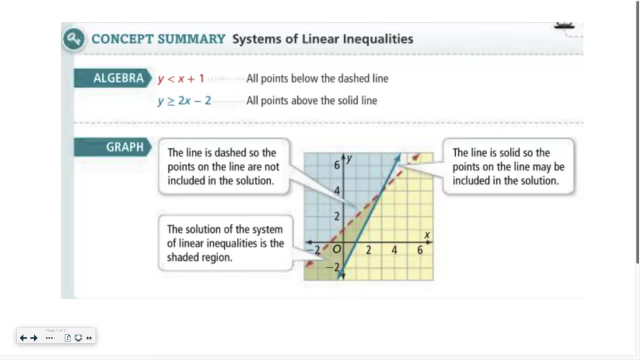 And that's okay. This is a special type of system. This is actually considered a no solution. Okay. When the shading does not overlap, there's no solution, Okay. So our concept summary for today is: the solution is always the overlapped shading. 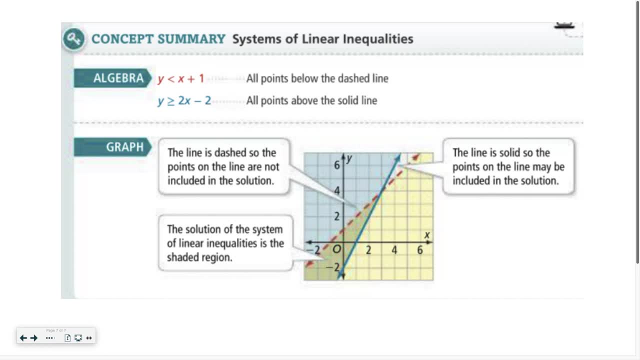 Okay, If you have questions about this or anything else, please be sure to reach out for some help And let me know I'm more than happy to help you. Have a great day.